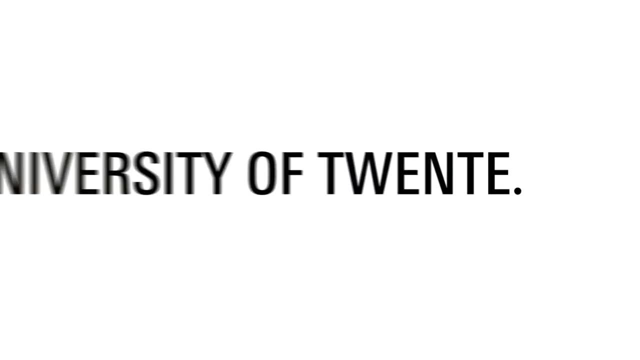 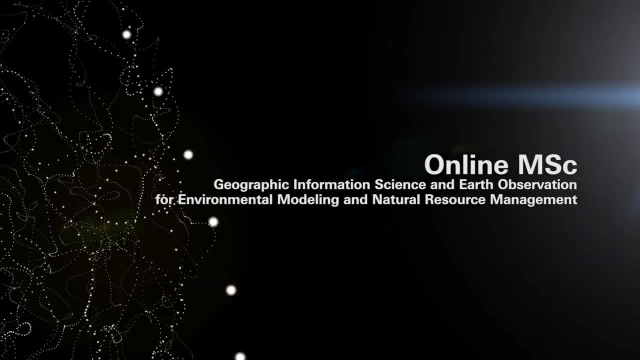 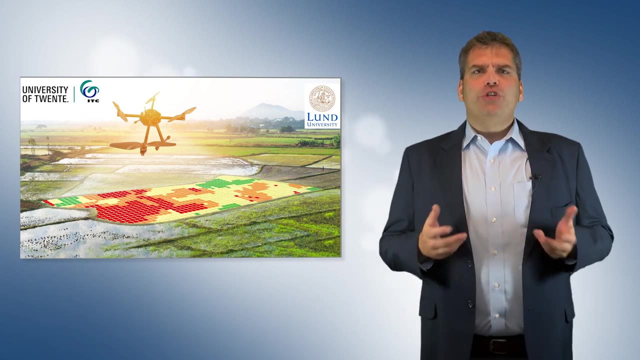 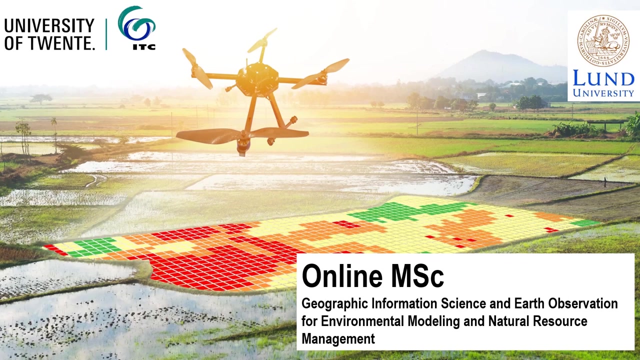 Hello everyone. Would you like to become an expert in the rapidly expanding field of geographic information science and remote sensing And, in the meantime, gain knowledge on topics such as food security, water management and climate change? Then the online MSC offered by both ITC faculty at the University of Twente and Lund University might be the right. 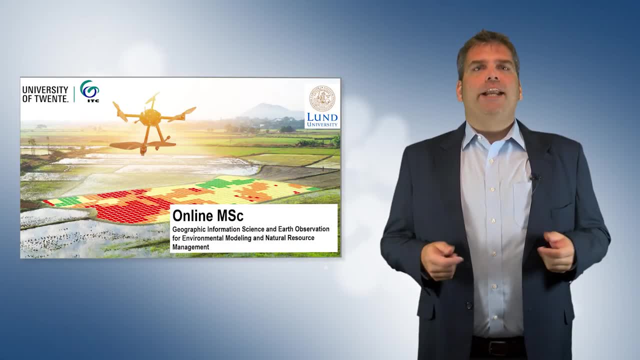 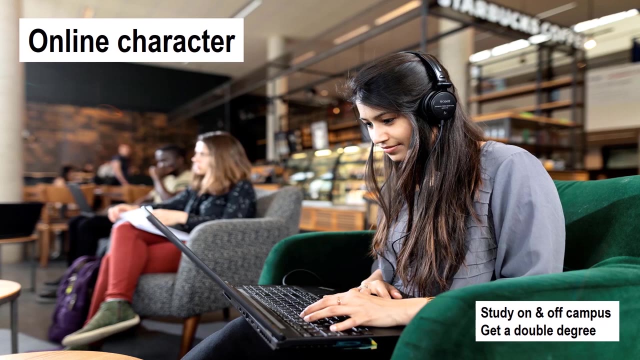 one for you. My name is Michael Marshall and I'm an assistant professor in the Department of Natural Resources in the ITC faculty of the University of Twente. I am also the teacher of today's mini lecture. In order to introduce you a bit to this online MSC, I will start. 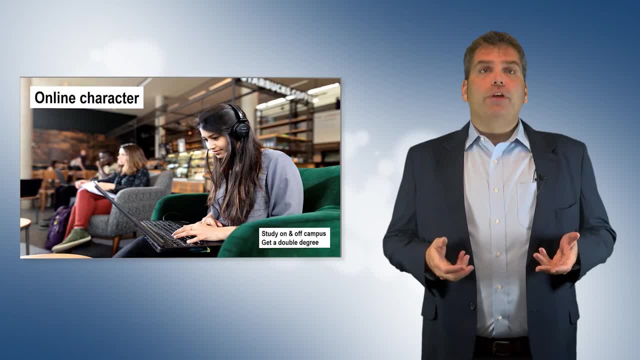 by highlighting the flexibility it offers. For instance, if you recognize yourself in a work-family lifestyle and you need flexibility in content, in study location and in study tempo, this might be the right choice for you. By following this online MSC, you can. 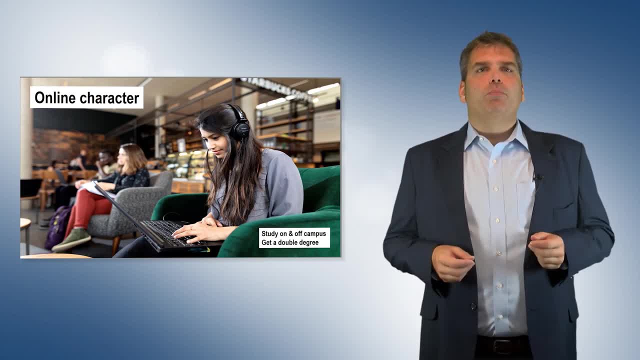 also get a double degree if you follow 25% of the program on campus, where you can experience the international environment of ITC. In the end, you will be awarded a degree from Lund University and a degree from the University of Twente, ITC. 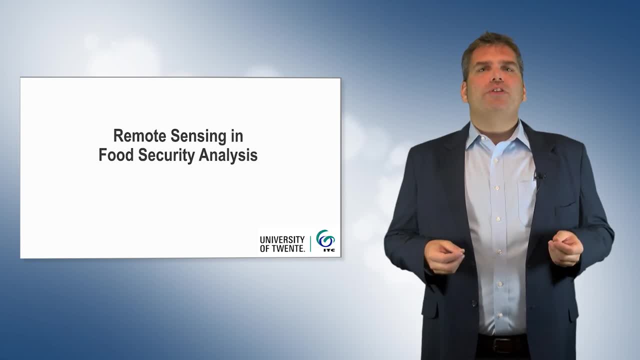 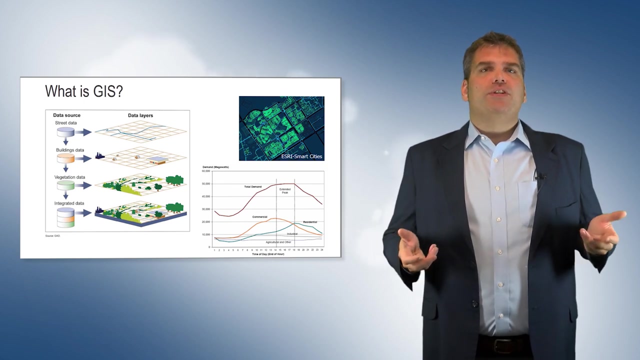 Today in this mini lecture, we will jump into the topic of remote sensing for food security analysis. Other courses covered in this online masters are electives from website: hydrology, computer programming, ecology, 5-6 example: internet GIS. GIS can stand for geographic information science or geographic information system, GI science. 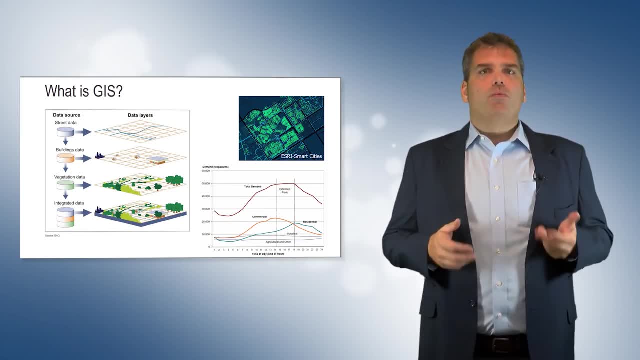 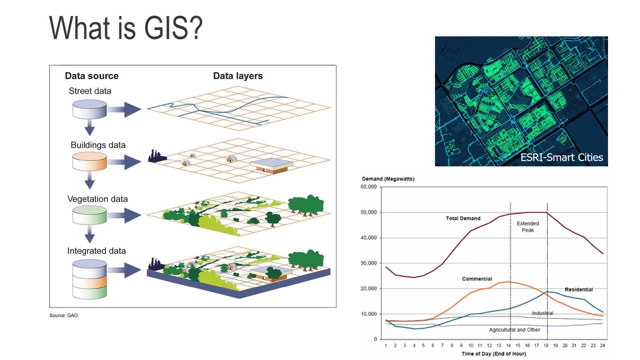 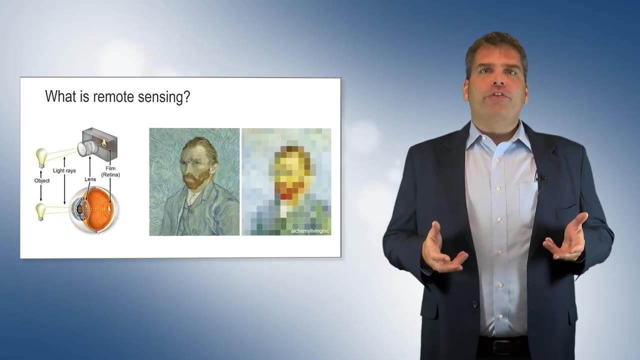 raises questions about geographic information systems. geographic information systems concerning the acquisition, processing, representation and analysis of geospatial data. Geographic information systems are tools that allow GI scientists to manipulate geospatial data. Remote sensing is an important category of geospatial data. A remote sensor can be defined. 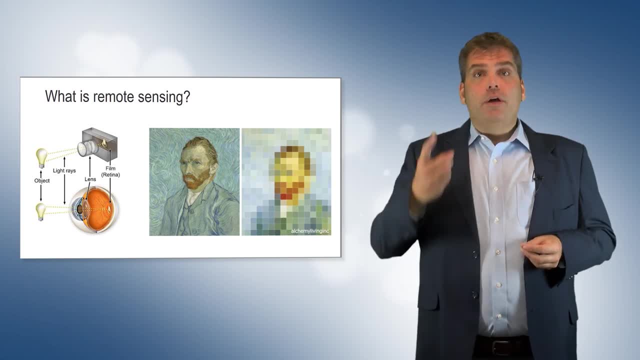 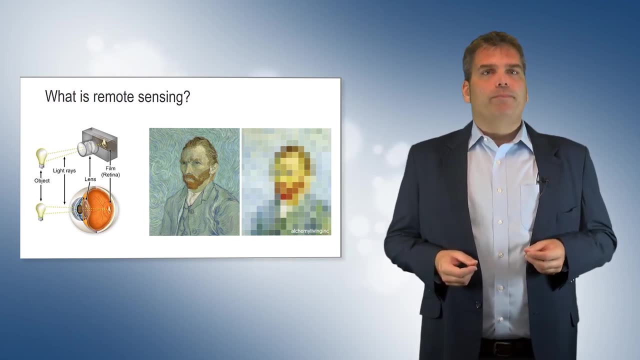 as any instrument that collects information without touching it. The human eye, for example, is a remote sensor because it receives light energy from the environment. It can also be used to detect energy from a source without touching it. The digital camera is a more. 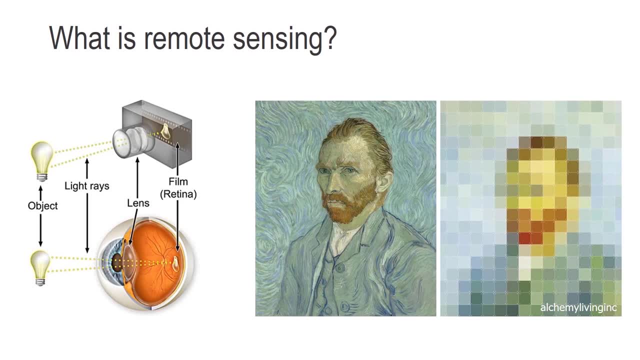 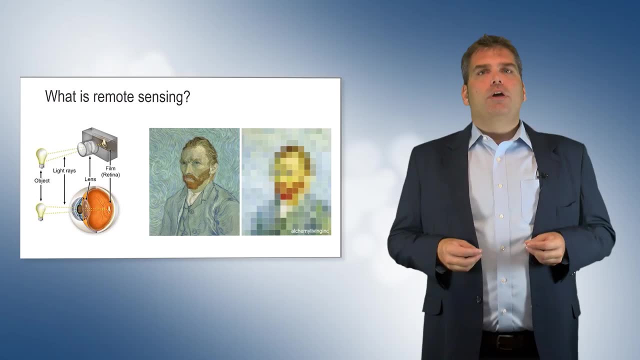 modern remote sensor. A digital camera records light reflected from a surface and stores it as an image. Digital images consist of pixels or grid cells. Light intensity at various frequencies of the electromagnetic spectrum are represented in each pixel by a digital number. Similarly, sensors on board satellites unmanned 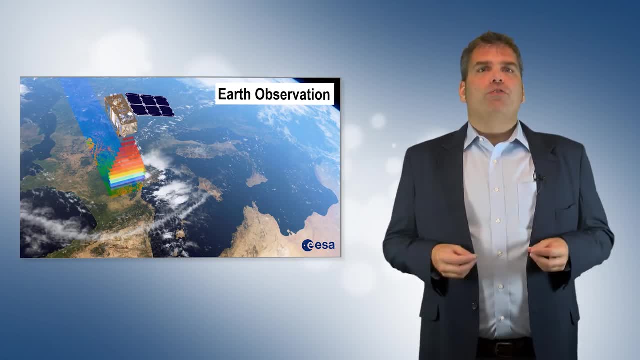 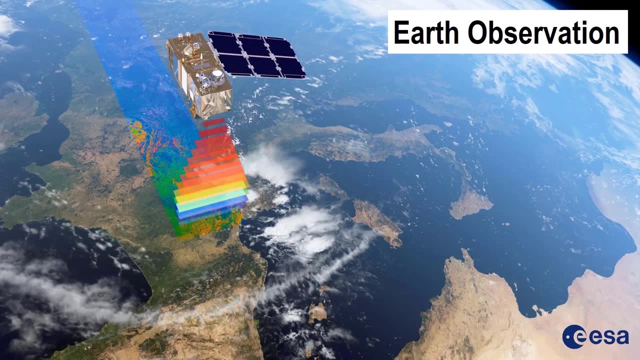 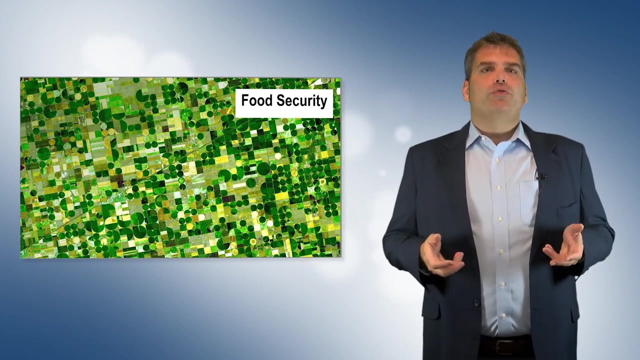 aerial vehicles or airplanes record light reflected or emitted from a source across the electromagnetic spectrum. They record current surface conditions and relay that information back to Earth. We call this type of remote sensing Earth observation. Let's take a brief look at how Earth observation is used for food security analysis. Food security- 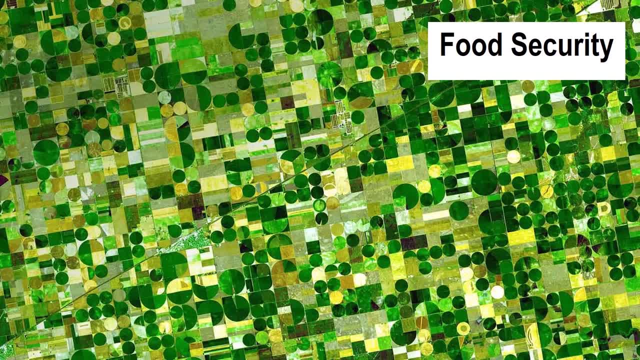 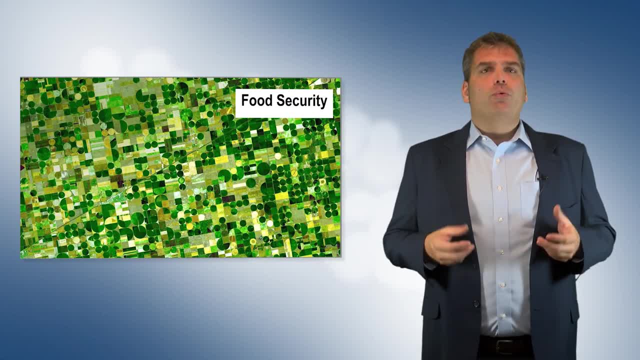 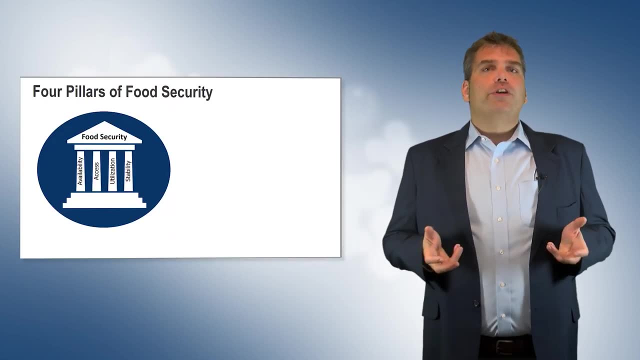 analysis determines whether individuals, households or other individuals are being households, communities or other populations are hungry and food insecure. It also assesses the underlying causes which are important for decision makers to design appropriate interventions. Food security can be evaluated by four metrics. 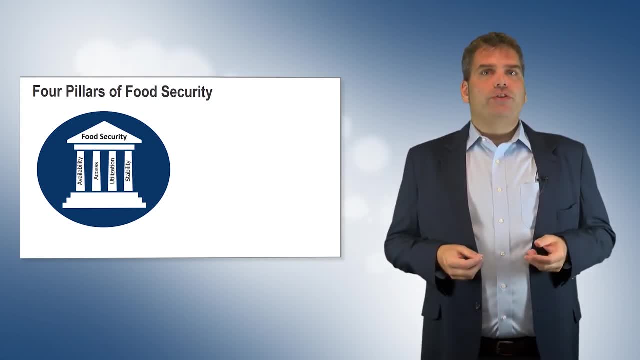 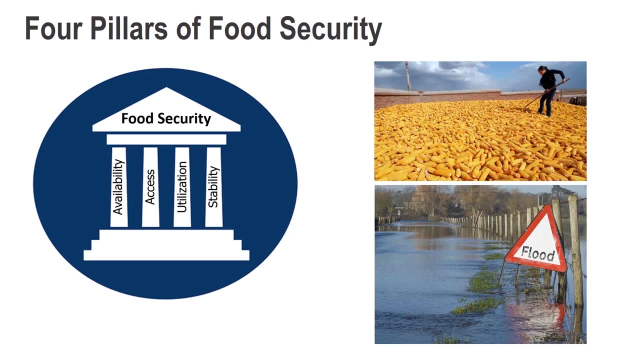 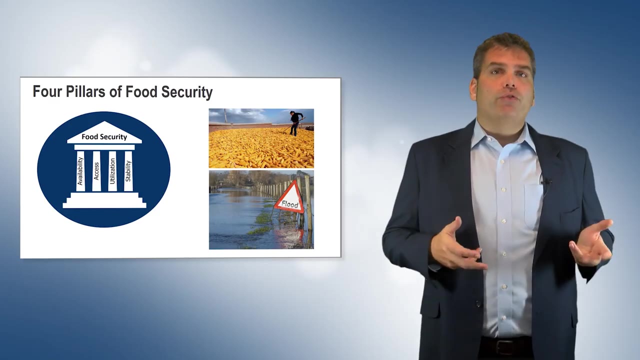 They are availability, access, utilization and stability. Availability deals with the supply side of food production. It not only concerns the amount of food produced, but whether food can be brought to market and exchanged for some form of currency. Droughts, floods, land degradation and poor infrastructure can greatly reduce availability. 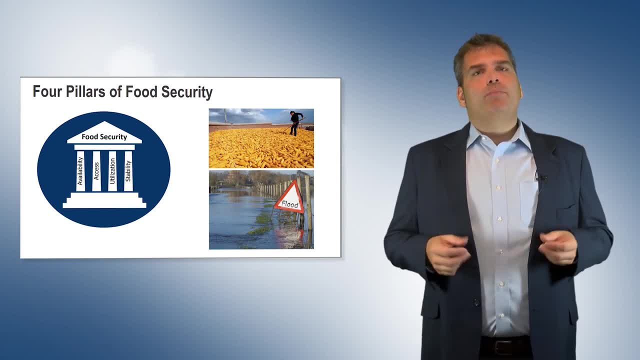 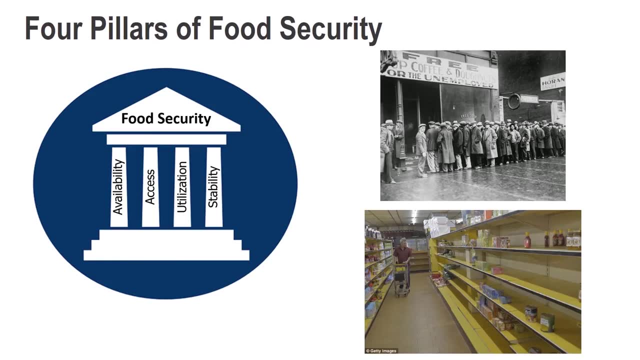 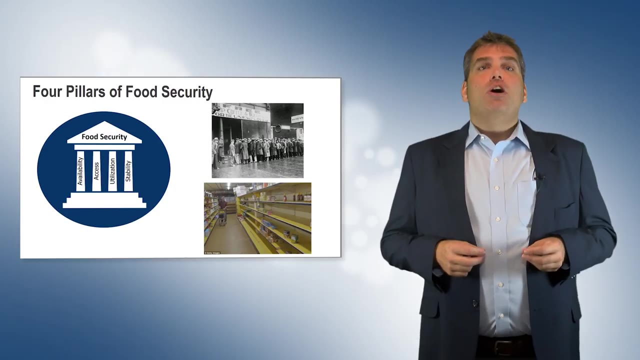 Access, utilization and stability represent the demand side of food production. Access refers to the purchasing power of a population. There can be an adequate food supply, but if the population is economically poor they cannot afford it. Price spikes due to local or global food shortages can prevent access to the world's 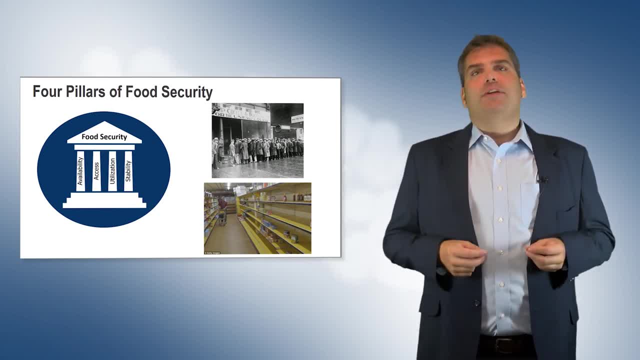 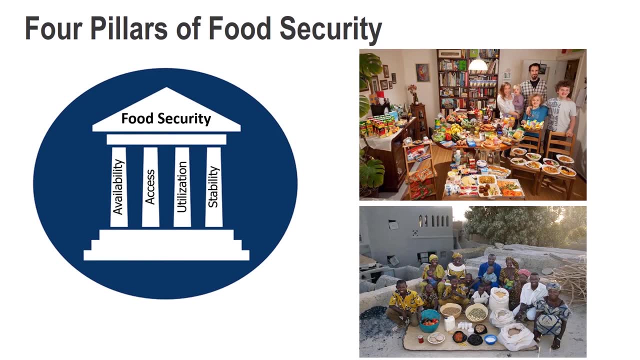 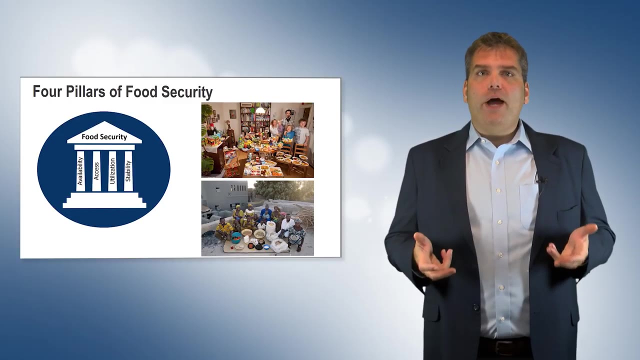 poor, while richer populations remain unaffected. Utilization deals with nutrition. It not only concerns which kinds of foods are consumed, but how food is processed and prepared. Fried processed meals consisting mostly of carbohydrates, for example, would be considered poor utilization. 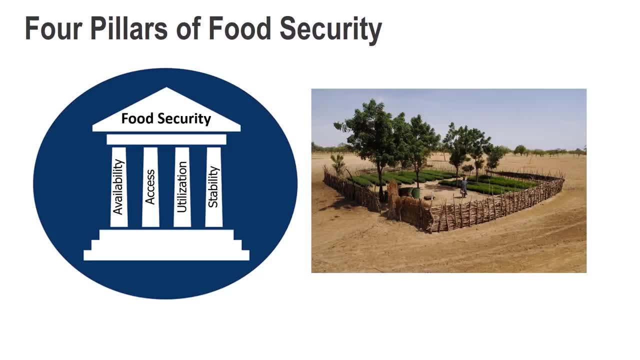 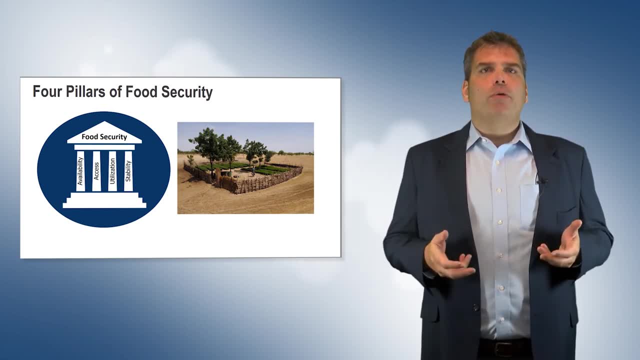 Last factor, stability measures the tendency and persistence of food insecurity over time. Chronic or permanent food insecurity is the most extreme form of instability. It is usually triggered by periods of infrequent food insecurity that slide a population further down into the poverty trap. 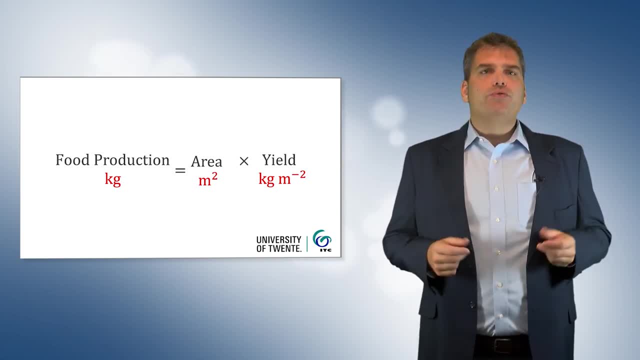 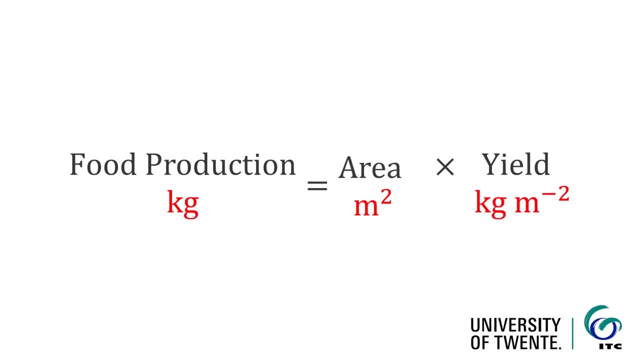 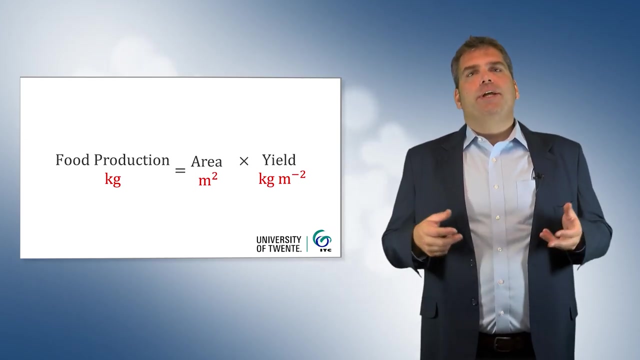 For food security analysis. Earth observation is almost exclusively used to estimate food availability. Specifically, the amount of food. Food production is defined as the harvested crop area multiplied by the harvested crop yield. It is typically measured in kilograms or metric tons. Crop area is measured in square meters or hectares. 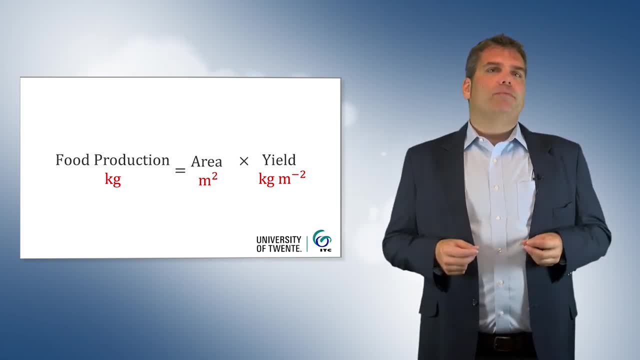 It is simply defined as the area over which a crop is harvested. In practice, however, It is difficult to determine because what defines a quote crop varies. Is crop area only the cultivated area, or does it also include infrastructure in uncultivated areas? 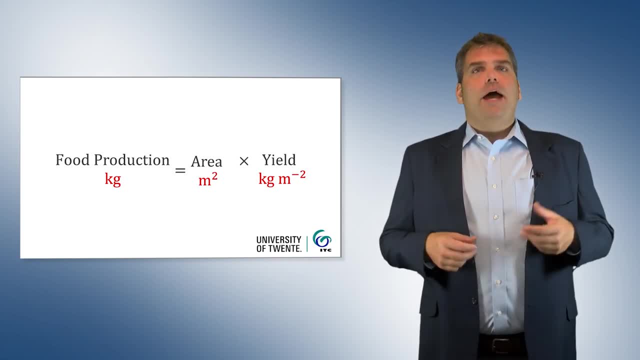 Should it be defined by the area planted or harvested? How should it be measured in mixed cropping systems or systems with more than one growing season, as is common in the tropics? Several remote sensing techniques have been developed to estimate crop area. We will discuss this later. 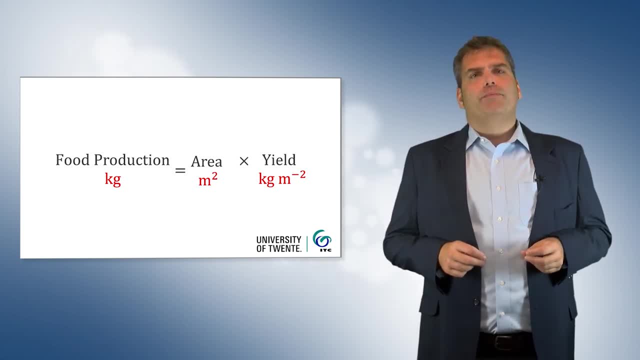 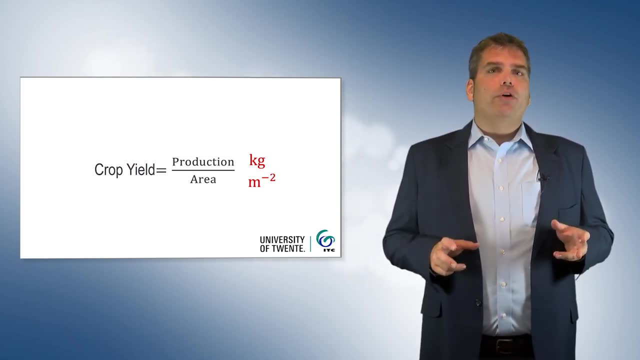 Thank you, Thank you, Thank you. By the way, let me share my screen. I only used this screen in my lecture and I will post these in a separate lecture. For now, I would like to focus on crop yield estimation. Crop yield is the ratio of the mass of grain, seed or other agricultural production to 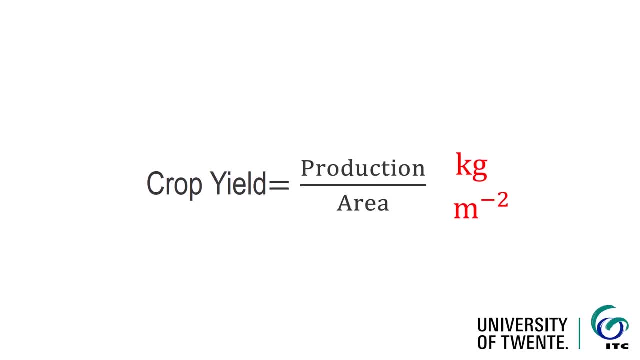 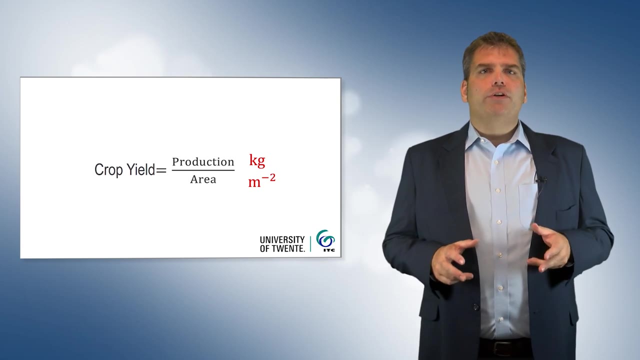 a standard area. Like production and crop area, mass is measured in kilograms or metric tons, while area is measured either in square meters or hectares. It is often confused with crop biomass, which is the total amount of crop biomass of above-ground material collected at harvest. yield is the marketable fraction. 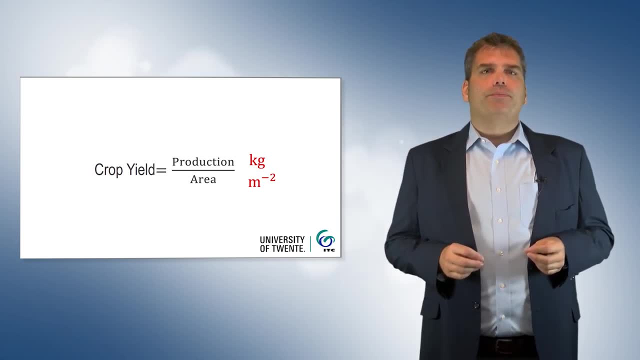 typically around 50 percent of crop biomass. the green revolution consisted of a number of critical agricultural achievements that increased crop yield and helped meet demand from a rapidly growing global population. of course, this narrative has many critiques and i would encourage you to study them in your free. 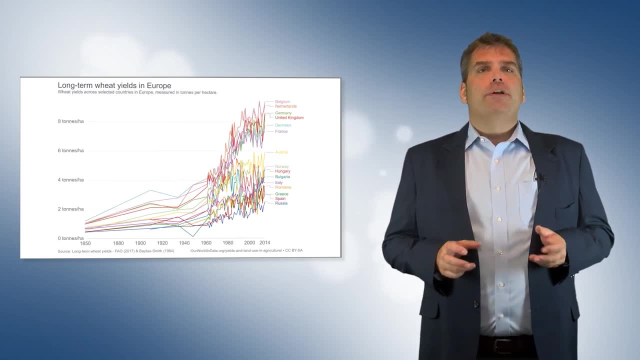 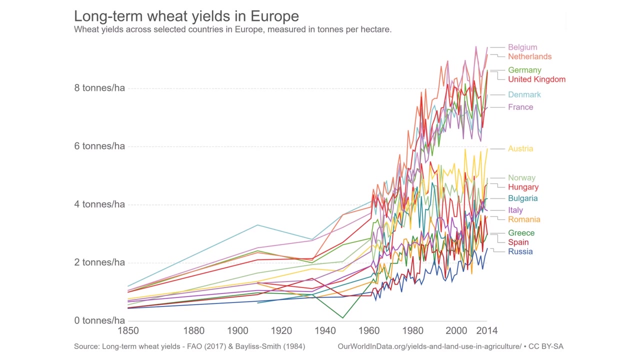 time. this chart tracks wheat yield in metric tons per hectare from 1850 to 2014 for several countries in europe. as you can see, the green revolution began in the 1930s, but it didn't really take off until the late 1960s. what made this rapid increase in production possible? 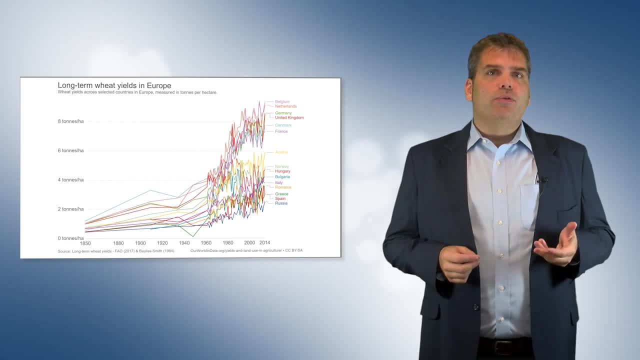 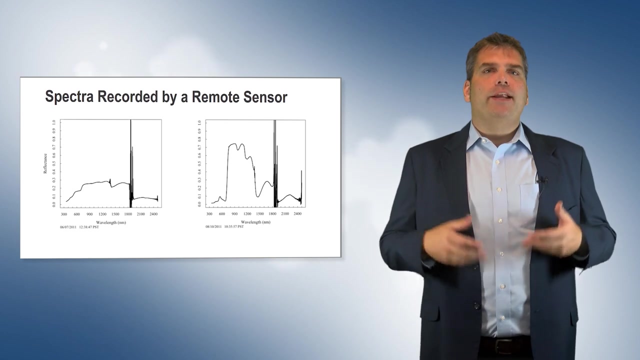 the expansion of arable land under cultivation and irrigation were perhaps the most important achievements. breeding crop. wild-bearing crops were also important, in which they helped not only to create top Location but also to provide More efficient crop production. crop yield models try to capture the factors of food production in order to better understand. 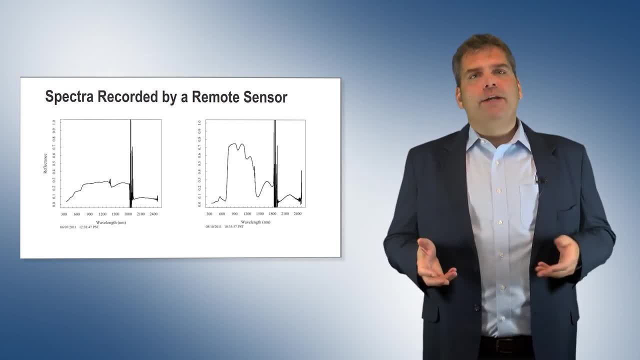 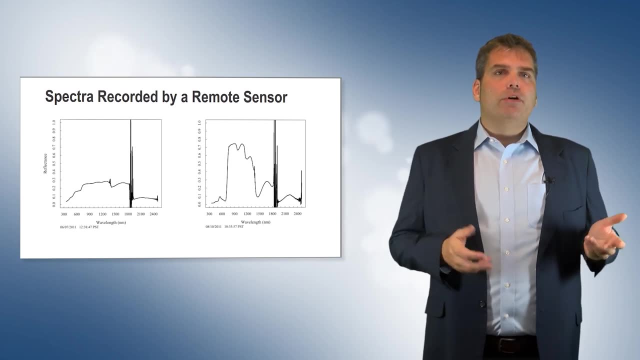 agricultural systems and to aid growers, farm managers and other decision makers in optimizing food production. whether empirical, semi-empirical or process-based models are important but are not always the best models for this process, so we have tried to increase the number of crop yield levels in the last 20 to 30 years. 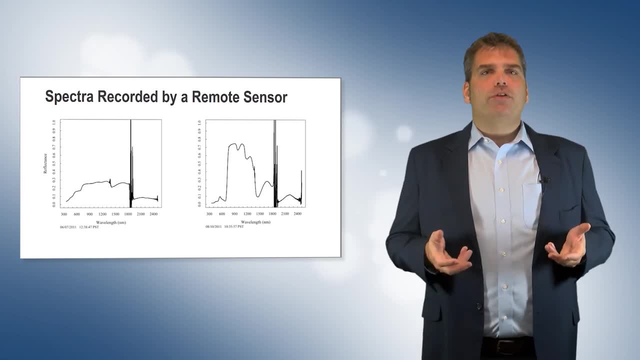 employed. spectral information collected by the remote sensor is used to develop a vegetation index. Perhaps the most famous is the Normalized Difference Vegetation Index, or NDVI. NDVI exploits the spectral properties of plants in the red and near-infrared or NIR wavelengths. 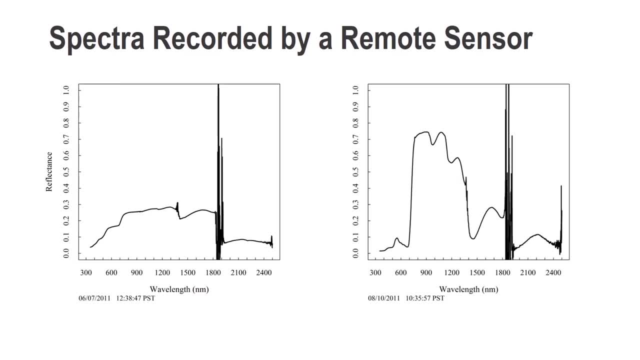 of the electromagnetic spectrum. These diagrams represent the spectral information recorded by a remote sensor above a cotton field in California for two periods of time. Peaks represent regions of strong reflectance, while troughs represent regions of strong absorption. In each diagram, focus on three regions of the electromagnetic spectrum. 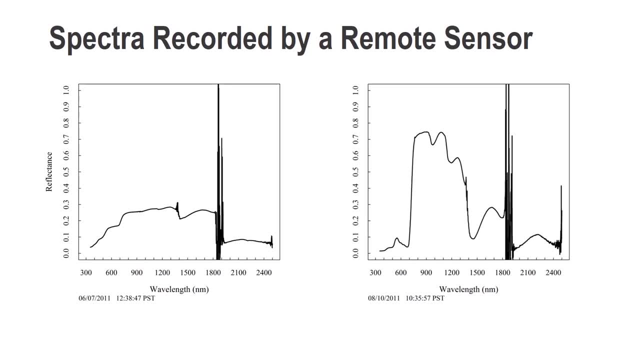 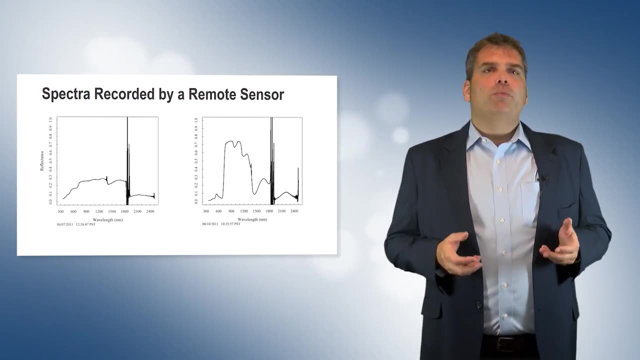 The green portion around 550 nm, the red portion around 670 nm and the NIR shoulder which begins around 780 nm. The first spectrum was recorded in June and represents the period when the cotton field is dominated by soil spectra because the cotton is just sprouting. 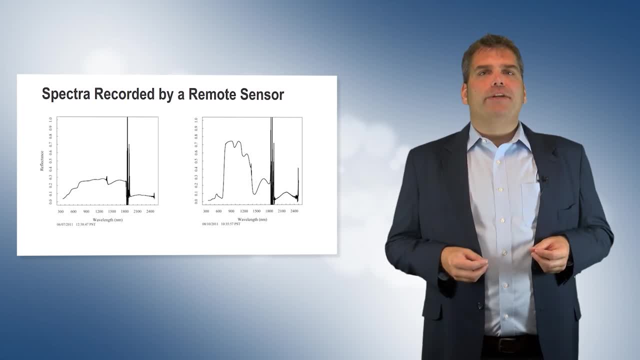 As can be seen, light across the spectrum is being mostly reflected In August, when the field is photosynthesizing and fully productive. there is an obvious peak in the green and NIR and trough in the red. The reflectance in the NIR is due primarily to the total amount of light that is released. 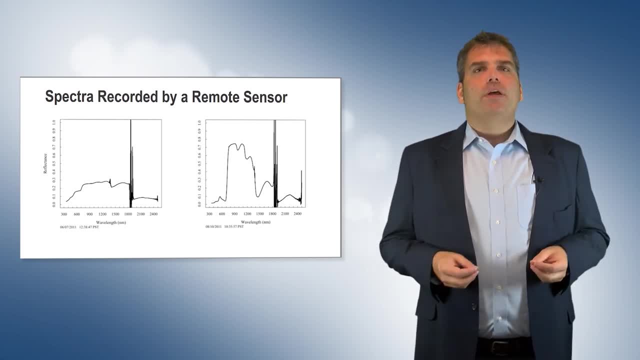 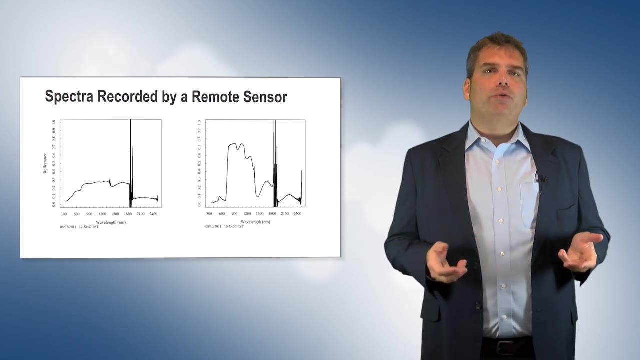 by the NIR primarily to the structure of cotton. NIR is not visible to the human eye, so we don't actually see it. It can, however, be detected by remote sensors. Crops absorb strongly in the red portion of the spectrum. Chlorophyll in plants which convert sunlight to food preferentially absorb. 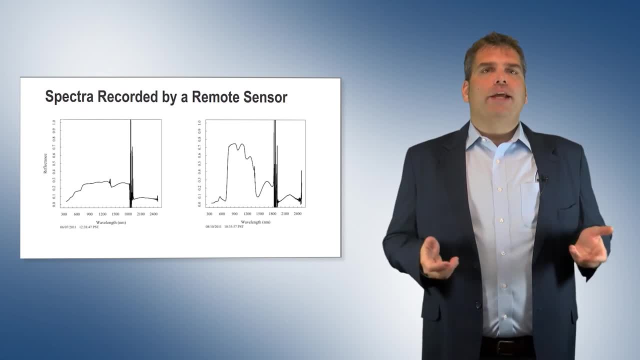 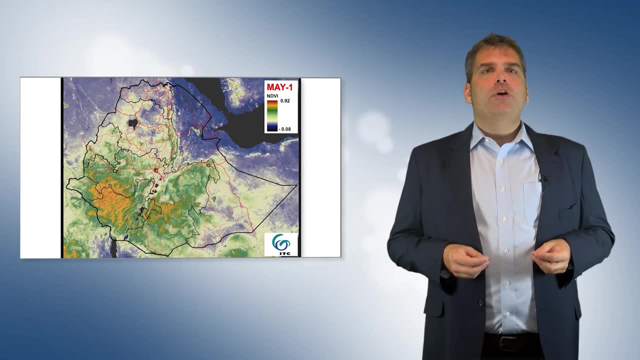 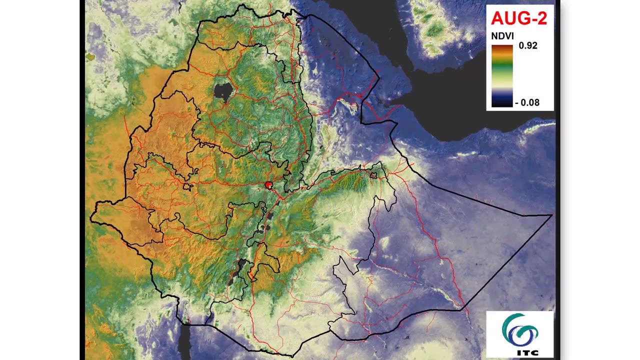 red light. If the cotton reflects more light in the NIR and absorbs more light in the red, NDVI increases. This animation for Ethiopia demonstrates an empirical crop modeling approach. We see NDVI derived from remote sensing over a year. It is sensitive to the greenness or 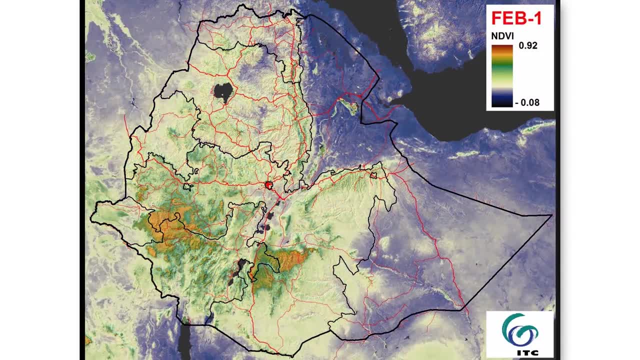 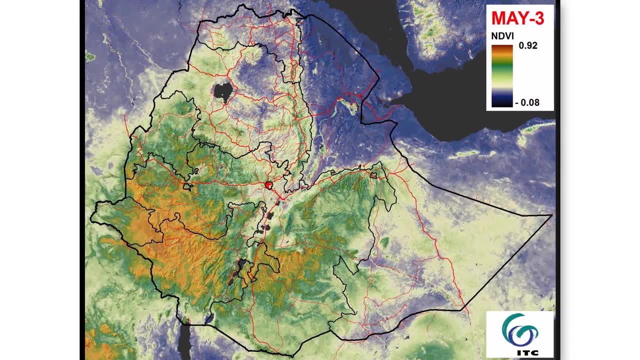 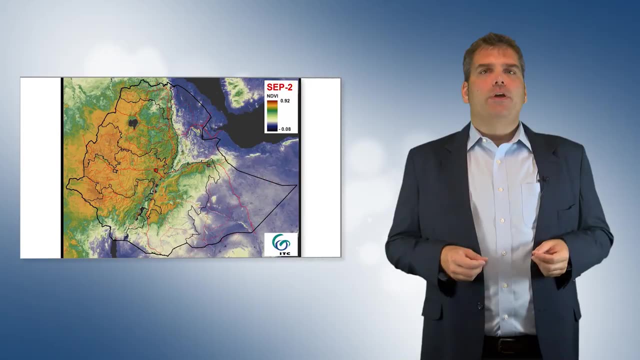 biomass of crops When NDVI is high. as can be seen in the agriculturally productive western and southern parts of the country from the beginning of May, biomass and productivity increase due to the onset of NIR. Images in this case are from Dr Keistabe at ITC. 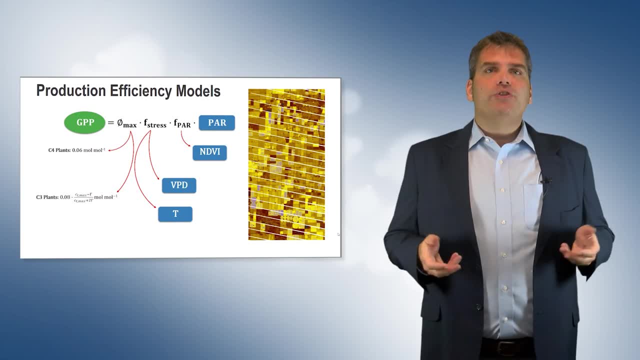 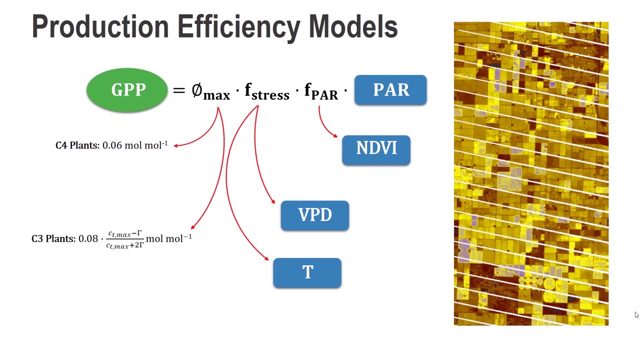 Semi-empirical models, also known as light use or production efficiency models, consist of cost functions that regulate the amount of biomass generated by a crop during photosynthesis. The functions typically relate to quantum efficiency or the ability of crops to convert CO2 into biomass. Temperature, vapor pressure and temperature are all related to biomass. 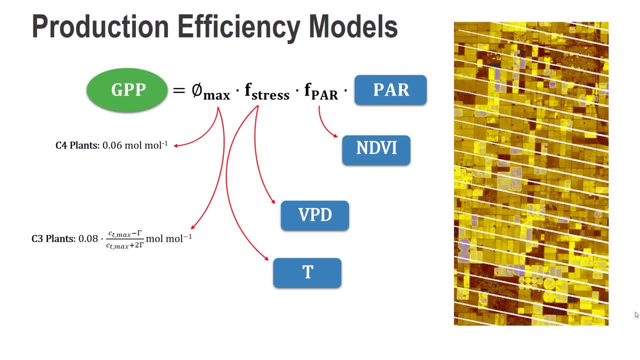 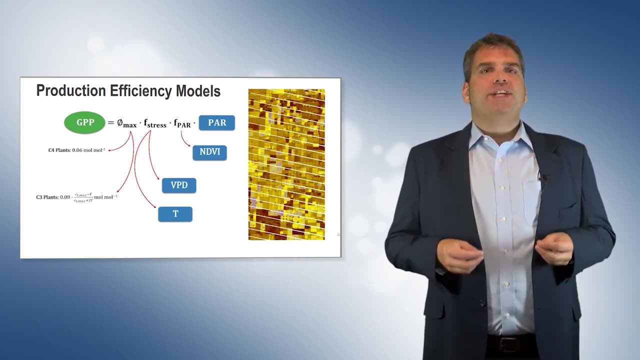 In this example we can see the temperature deficit or relative humidity and the amount of energy available from the sun, or photosynthetically active radiation, also known as PAR. Photosynthesis is the process by which crops convert sunlight into food and then biomass. Remote sensing. 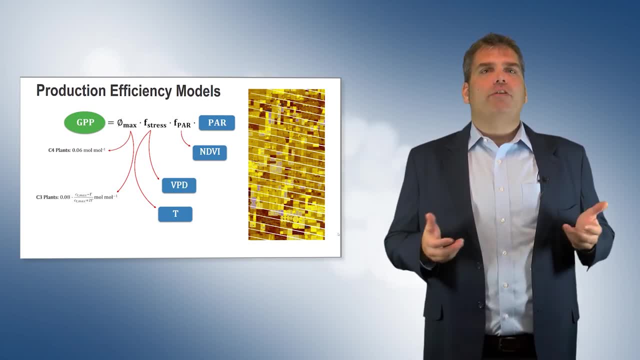 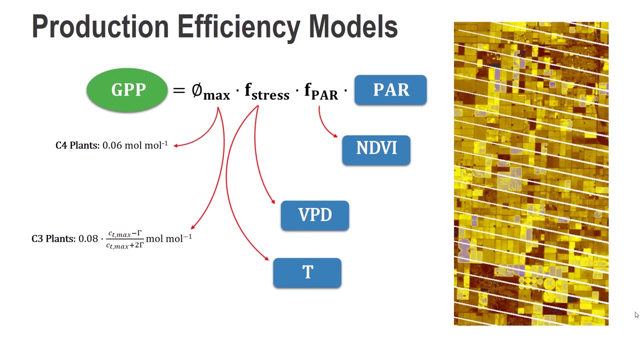 data are used in production efficiency models to derive the fraction of PAR or the leaf area index LAI. F-PAR and LAI essentially measure the fraction of sunlight that is used by the crop to make biomass. The diagram on the right uses Landsat imagery to predict yield in this way at 30 meter. 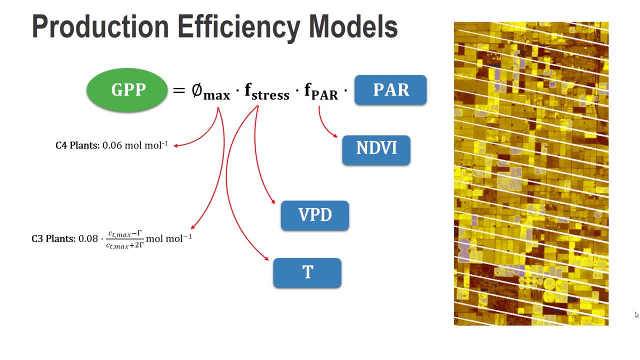 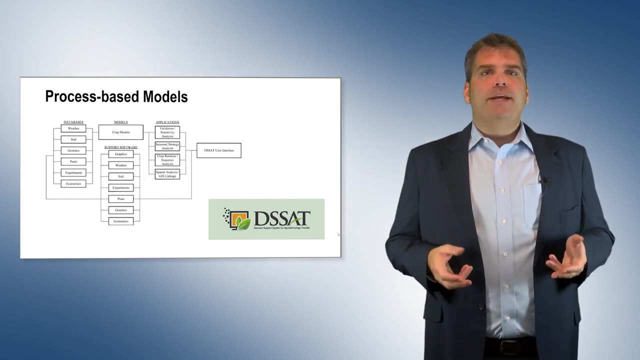 resolution. Areas in bright yellow are more productive than areas that are a duller yellow or brown. The white striping is emblematic of Landsat 7. ETM+. Process-based models use a number of empirical and theoretically based relationships to estimate crop yield. In addition,